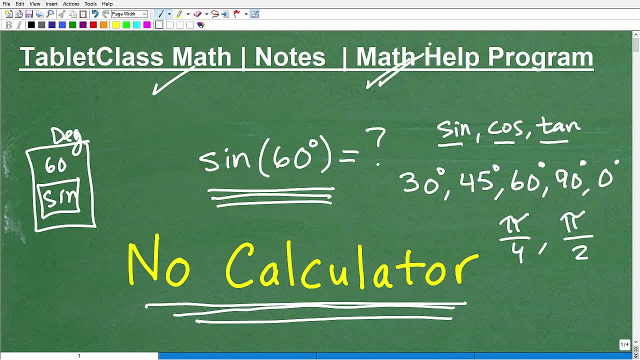 what I like to believe is one of the best online math help programs there is. Of course, I'll let you be the judge of that. You can check out my math help program by following the link in the description of this video, But basically I'm going to show you how to do that, So if you're 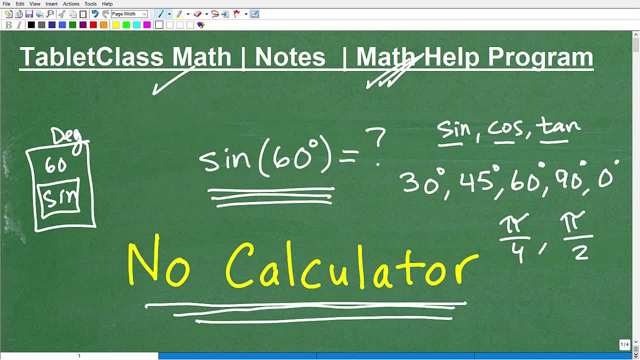 interested in learning more about math. you can check out the link in the description of this video. I have a hundred plus different math courses, ranging from pre-algebra, algebra one, geometry, algebra two. I'm going to be launching pre-calculus here shortly, which has all my advanced 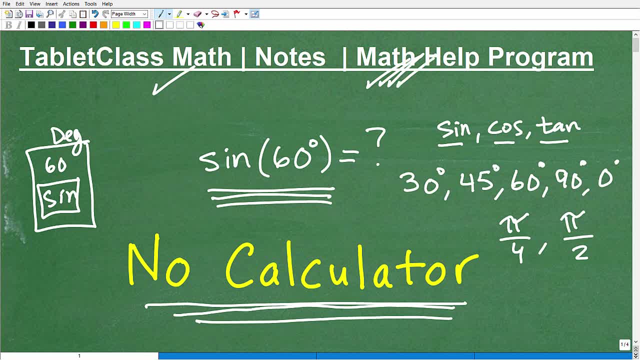 trigonometry in it, So I'm pretty excited about that. But I also do a lot in the area of test preparation. So if you're studying for the SAT, ACT, GED, HiSET, maybe the CLEP exam, 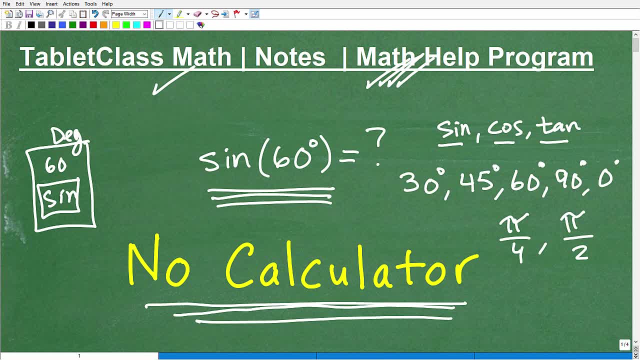 ACCUPLACER, ALEKS, teacher certification exam. all those exams have a lot of math on them. So if you don't have the math section, you don't do well on the exam, And of course we don't want that to. 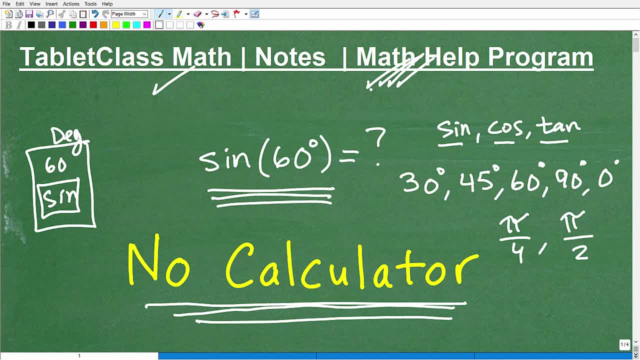 happen. So if you need help, just go to my website and check out my full course catalog. If I don't have the exam that you're studying, drop me a line and I'll help you out the best I can. I also work. 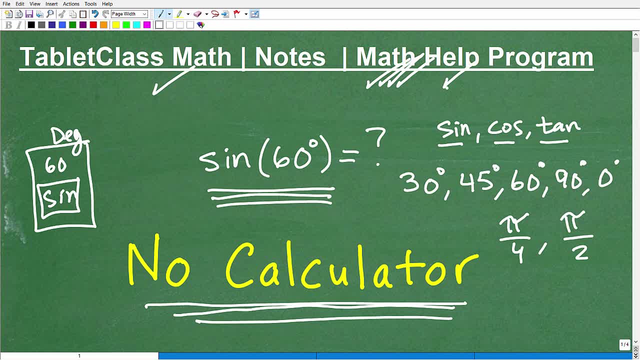 a lot with independent learners, like homeschoolers. So if you homeschool, I have a great homeschool learning program, And then obviously I help those of you that are struggling in your current math course. So, but one thing I can't do for you that you've got to do for yourself if you're truly 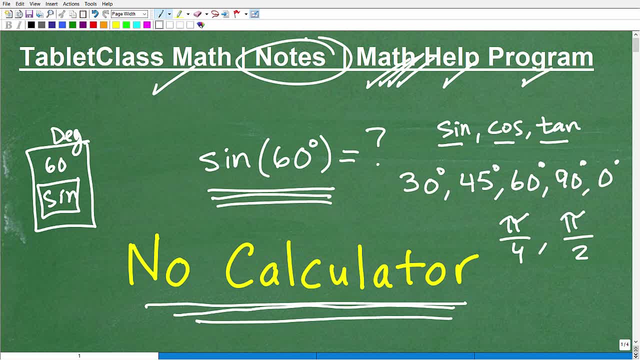 serious about improving and learning math, that is taking great math notes. So over decades of teaching mathematics, one thing is apparent to me: those students who have great notes, you know like, wow, your notes are amazing, Guess what They always get like great grades, No surprise. 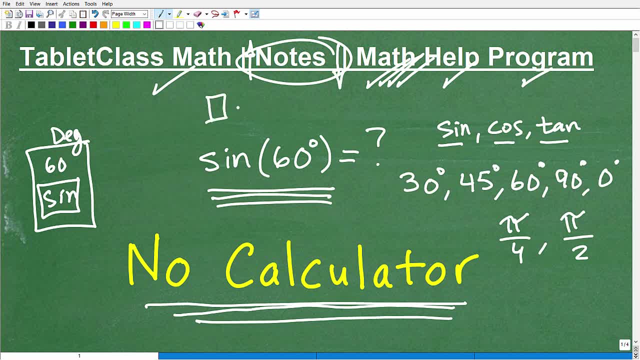 there, And the reverse is true. Those students who like to look at their cell phone, talk to their friends and maybe do their homework for another class during math class, And you'll be like, really People do that? Yes, In fact, a lot of students do this. 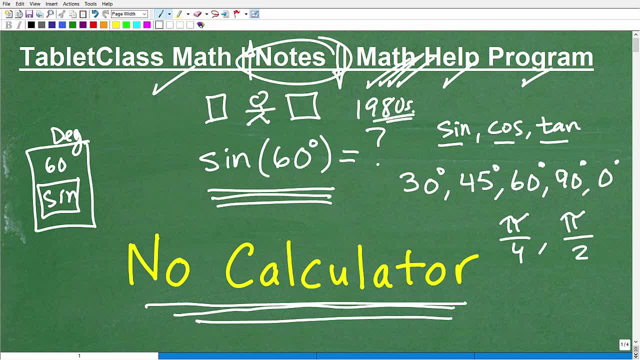 As a matter of fact, I did a lot of this stuff way back in the 1980s, except for the cell phone part. We didn't have that. But I was quite distracted And of course my grades look like this: C minus. And you know I'm like: listen, I get it. You know, as a teacher, you see things. 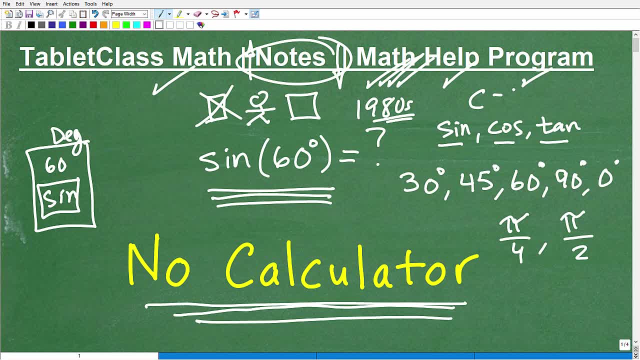 But if you really, really want to do well, you can't say, oh my teacher, you know I don't like my teacher, et cetera, et cetera. You've got to take responsibility for your learning, Okay, And? 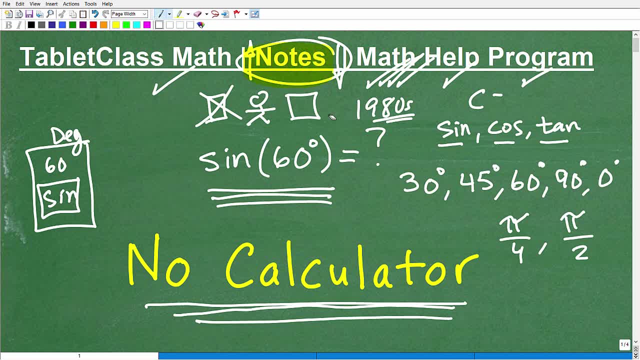 the biggest thing you can do to help yourself is to remain in the classroom, And that's what I'm focused and engaged on in class. Okay, And the best way to do that is to take great math notes, kind of really work hard at that. But as you're improving, I offer detailed, comprehensive math. 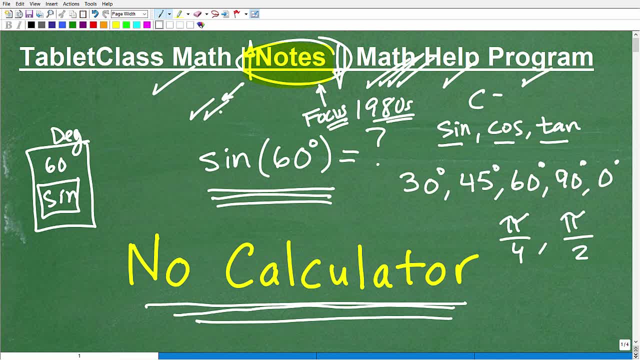 notes. So you got something to study from to include pre-algebra, algebra one, geometry, algebra two and trigonometry. You can find the links to those notes in the description of this video. Okay, So if you want to kind of play along here for a second and get your calculator out, 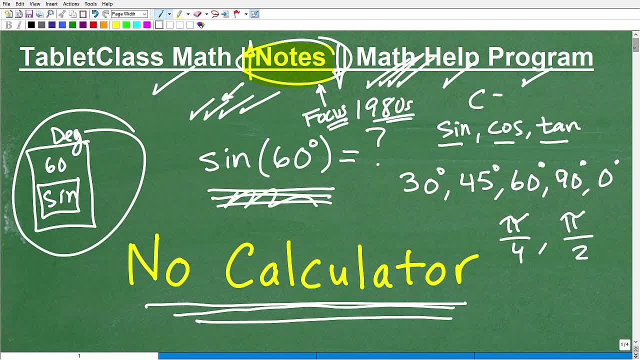 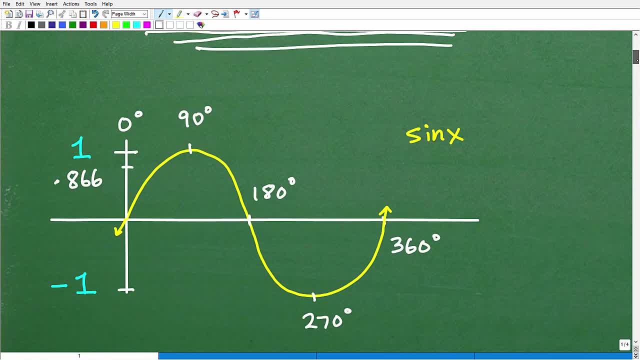 and figure out what the sine of 60 degrees is. you can. you know. that's good, That's fine, because you're going to be using your calculator and you'll get some sort of decimal value. Now let's take a look at the sine graph Now. 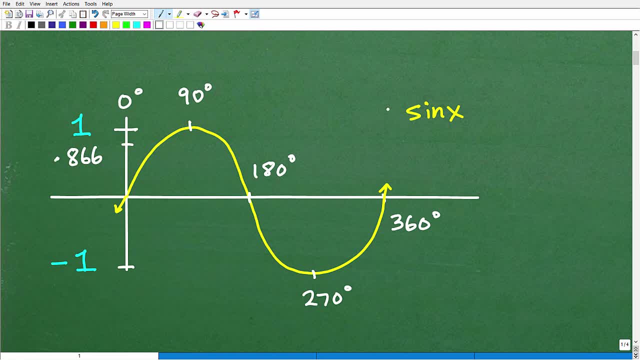 I don't know if you're familiar with this or not, but the graph of sine okay looks something like this: Matter of fact, it goes like this, over and, over and over again. It's called. that's kind of terrible, but basically it's a wave, Okay, A sine wave, And it's what we call a periodic function. 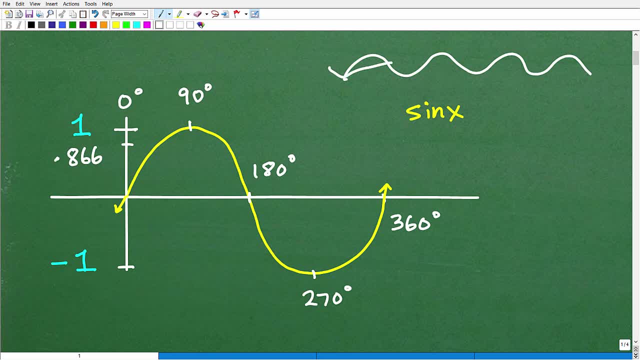 All right. It just kind of keeps repeating itself consistently And it bounces from one to negative one. This is the standard graph of sine x. All right, So y equals sine x, but you kind of get the idea. And this is what. 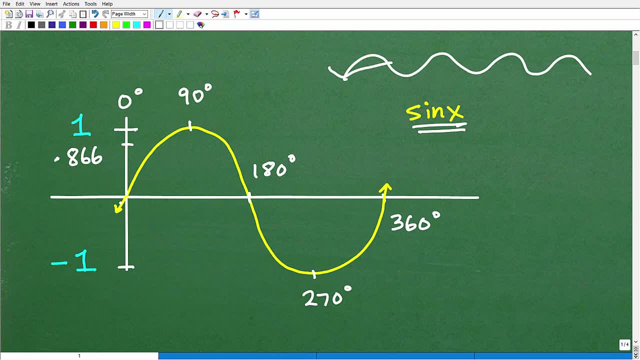 we call one period, one kind of yes, well, one period, one cycle okay, of the graph. Now kind of not doing it here correctly, but you can kind of see it here exactly Now. it starts at zero degrees, Okay, And at zero. 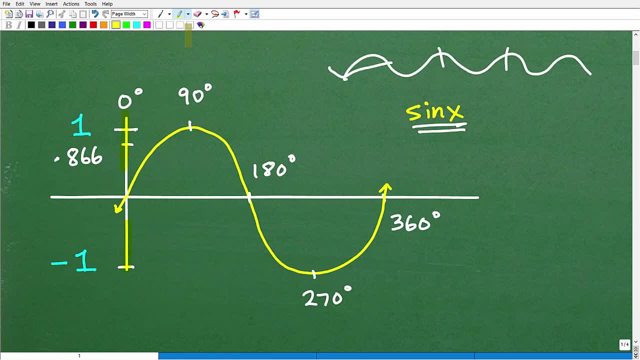 what you're looking at is this axis right here. Okay, So at zero degrees. this is degrees. Let's look at the yellow graph. Sine is zero. Okay, So at 90 degrees, as this sine graph is going up. 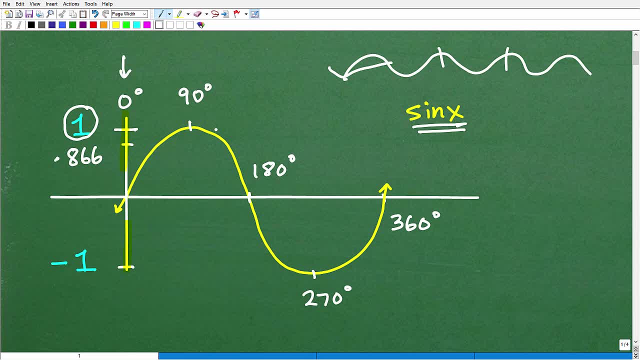 this is 90 degrees, Sine is positive one, Okay. Then the graph is going to go back down and then, halfway through, Matter of fact, just one cycle, Okay. One period here is 360 degrees, Okay. Or two pi radians, That's a different story, And you've got to be able to. 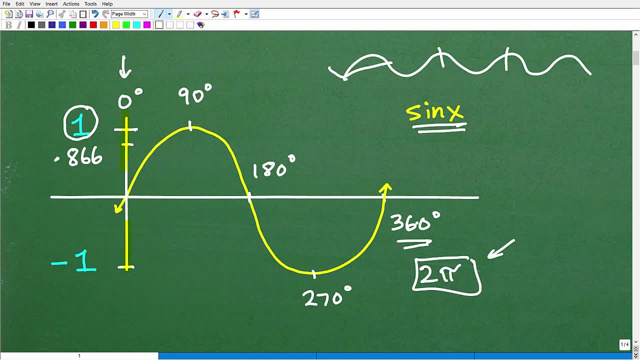 understand this basic sine graph and radians, But let's just look at it as degrees, because that's what we're dealing with, So let's continue on. So the sine graph at 180 degrees goes back down to zero. Now it's going down, And at 270 degrees it's at negative one. Okay, So there's negative. 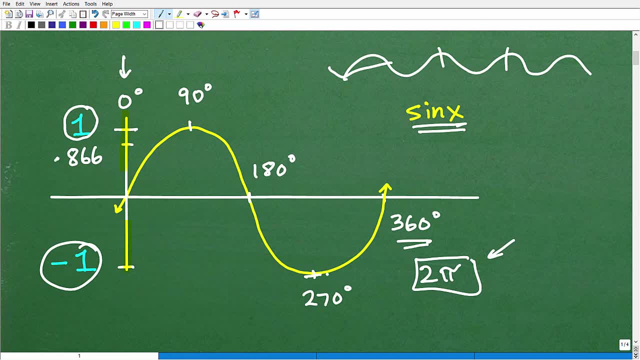 one. That's the value at 270 degrees. So you can see that the sine graph is going down And at. If you want to go into your calculator and type in, you know, sine of 270 degrees, you'll see it's going to pop out negative one. Or the sine of 180 degrees. you'll get zero. Or the sine of. 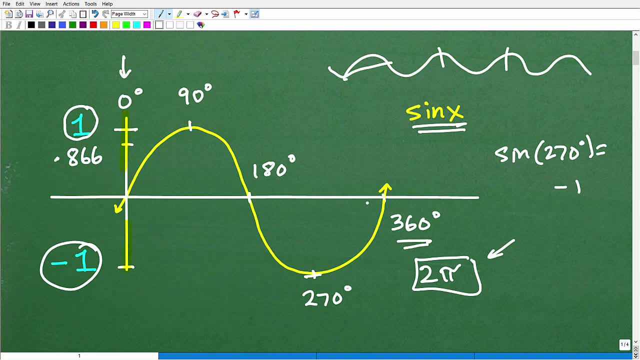 360 degrees, you're going to get zero again. Okay, So you need to be able to interpret these graphs. So graphs in mathematics are so important. Now let's go ahead and just try to estimate where the sine of 60 degrees is going to be. So if 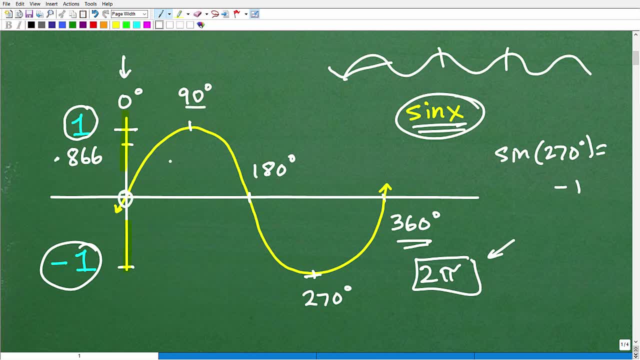 this is 90 degrees and this here is zero degrees. well, 60 degrees will be, maybe something like right here. Okay, so this is 90 degrees, right here. So 60 degrees would be like, say, right there. So what would be the value of it? Well, it's going to be less than one, because 60 degrees 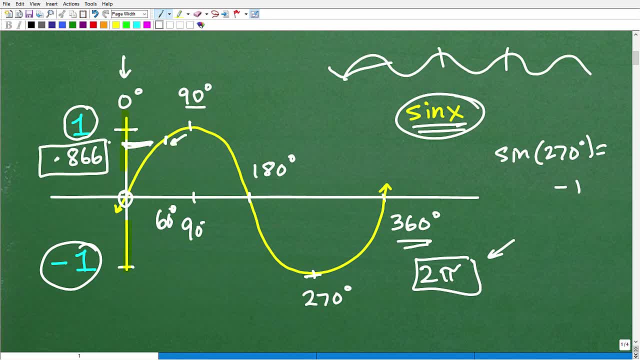 is less than 90. And actually if you go into your calculator, like I said, it's going to be a decimal around 0.866.. Okay, So if we go into our calculator and we go- let me get rid of this stuff here- And we go sine. 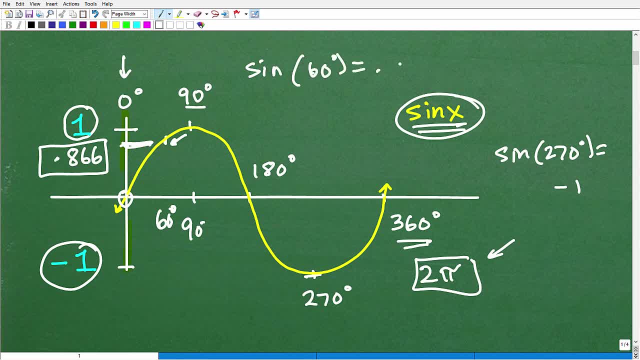 60 degrees, you'll get a decimal of like 0.866.. And there's some other stuff, but this is good enough for what we're doing here. Okay, but you can kind of see this graphically what's going on. 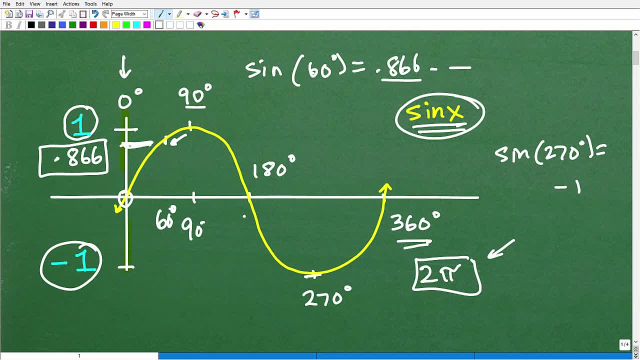 Now you need to be able to have a very good feel for the graphs of trigonometric functions. okay, as you study trigonometry, But anyways, there's another way we could approach this. you need to know this graph, but this is not the way we would actually find the exact value of the 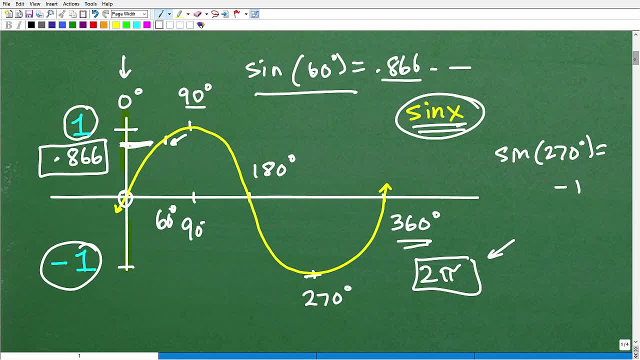 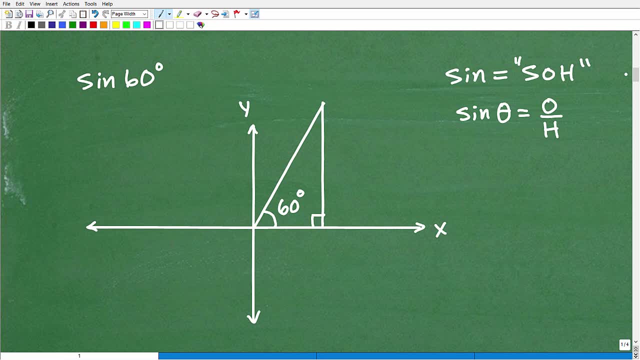 sine of 60 degrees And because I'm going to show you this right now. Okay, so this is what you want to do, right, you want to create a nice little reference triangle, Alright. so when you when an angle is what we call in standard position, it starts right here on the x axis and it goes. 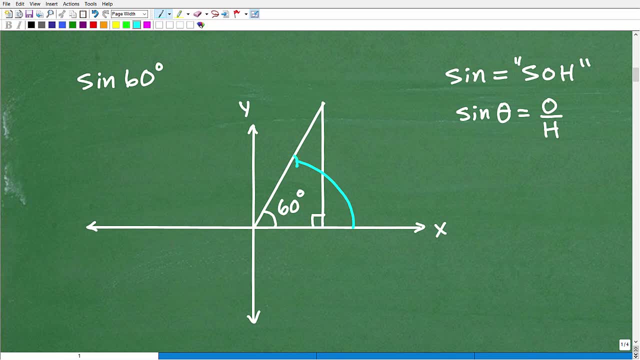 counterclockwise. Okay, So it goes this way, to its terminal axis, this way. So this is kind of its starting position, this is its ending position. So when we create an angle, you always start this way, a positive angle, right? So if I said plot 120 degrees, that would go past 90 degrees. this is 90 degrees. 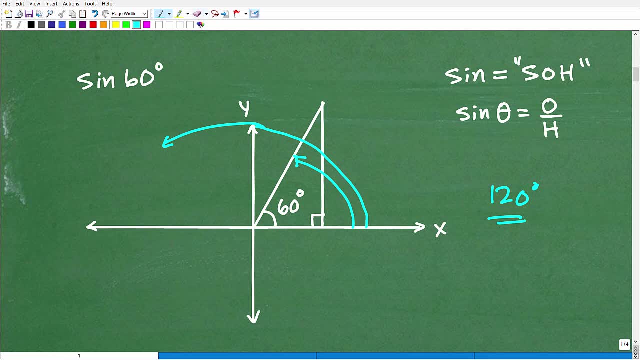 and you would continue on to 120 degrees, Okay. so hopefully that makes sense. Again, I'm kind of covering this pretty quickly here, But 60 degrees would be like right here. Okay, so it starts here and then ends there, So we would draw a nice little. 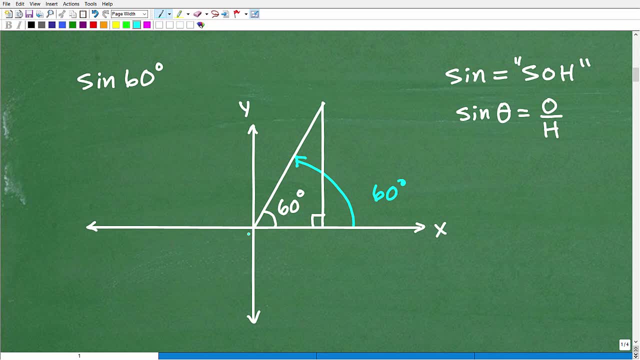 hypotenuse, starting or emanating from the origin. Okay now, hopefully for the most part, those of you out there watching this video going: okay, I understand that. Now what you have? okay, let me kind of put that in right there. So here is our nice 60 degree angle, And we want to 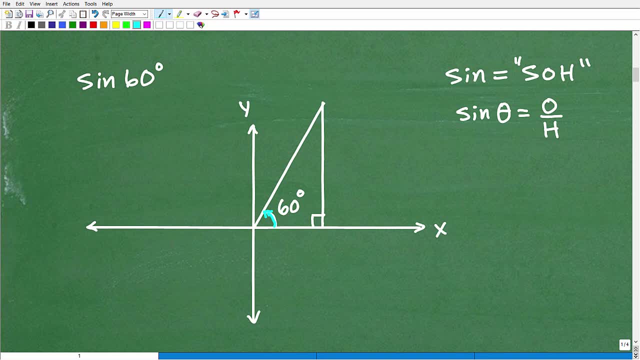 find the sine of this 60 degrees. So how do we do that? Well, we, first of all, we need to know the definition of sine. Okay now, if you remember from your basic trigonometry, you have this thing called: 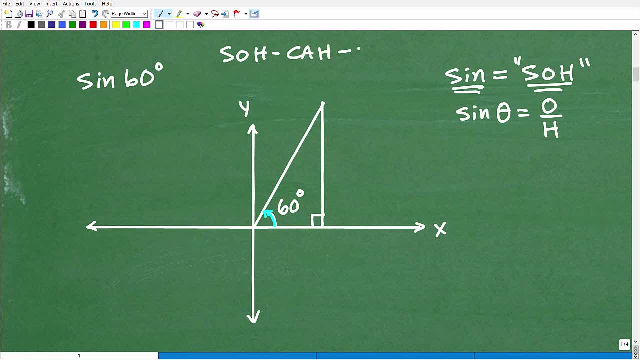 Soka Toa. Okay, now, if you are not familiar with this little phrase, you can check out more of my videos in my geometry playlist on basic trigonometry. Okay, basic right angle trigonometry, But you need to be familiar with this. Now, if you're not familiar with what's. 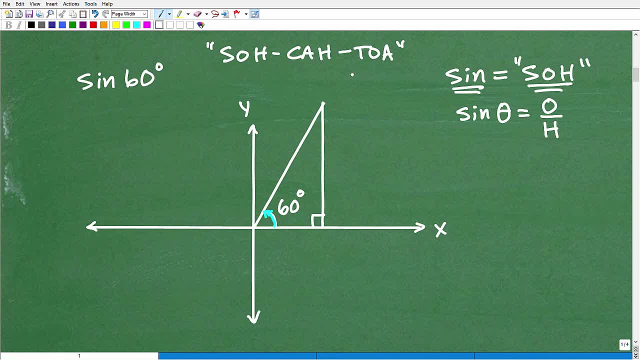 what is sine, what is cosine? then maybe this video is not the right one for you right now, But just let's play along here and continue on, Because the sine, this so part- we're talking about the sine. the, this, the co part, is talking about the cosine, and then this is talking about: 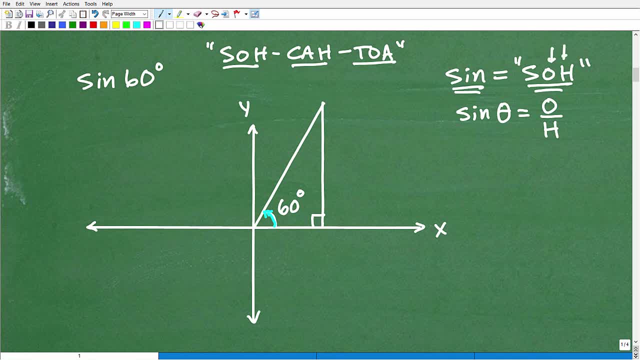 the tangent. So the sine this O and H, the sine of an angle, is equal to the hypotenuse over, I'm sorry, the opposite over the hypotenuse. Okay, now, here is our angle, right here. All right, the hypotenuse is always going to be the longest part of this right triangle. So there's. 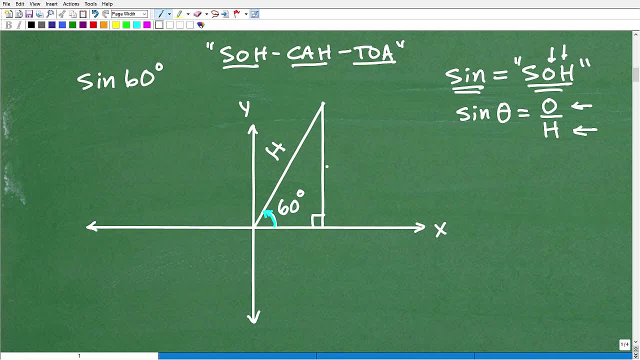 our H. So what's the opposite angle here? Okay, though, the opposite angle is this angle right there, And this is the adjacent angle. So we have an A and O and H, and you kind of figure out the rest of these ratios for these trigonometric functions When you kind of put in: hey, okay. 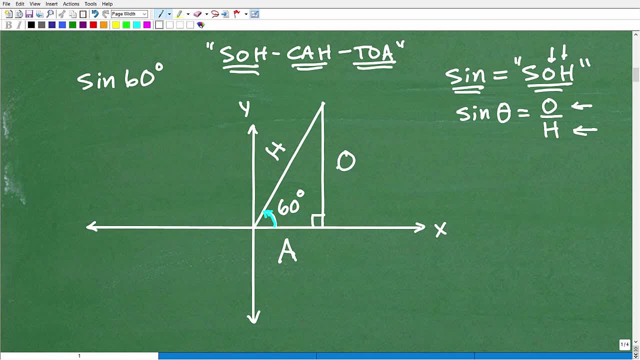 where's the hypotenuse, Where's the opposite, Where's the adjacent? You got to be careful, because the opposite and adjacent. you got to really think about where the angle is located, because if the angle is located here, this would be the opposite. Okay, but anyways, hopefully this makes sense. So the sine. 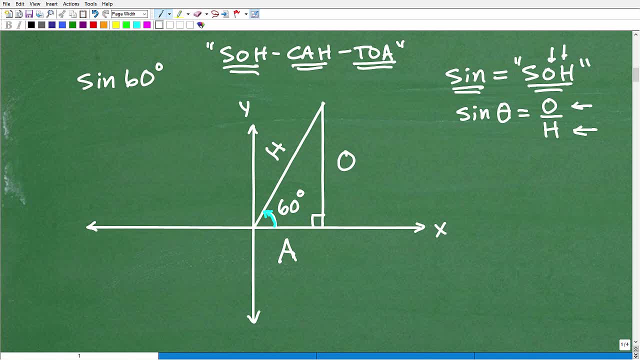 is equal to this. so which is the opposite over the hypotenuse. So in this case, right here, the sine of 60 degrees is going to be equal to this: O over H, this over, I'm sorry, this, this, right here, this line. 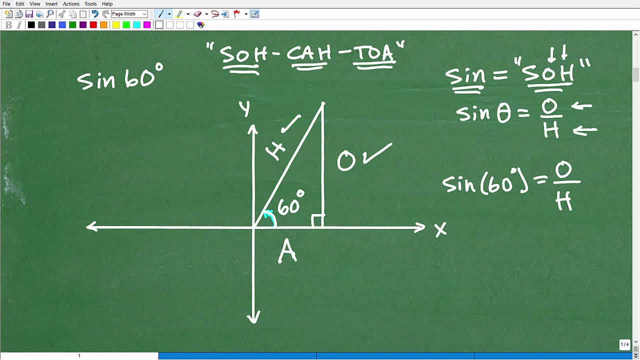 Okay, so now we need to figure out, well, what are those lengths? Because we can't answer this question unless we know those lengths. Well, luckily, we do know those lengths And this is going to be incumbent upon you really understanding special right triangles. There's two you need to. 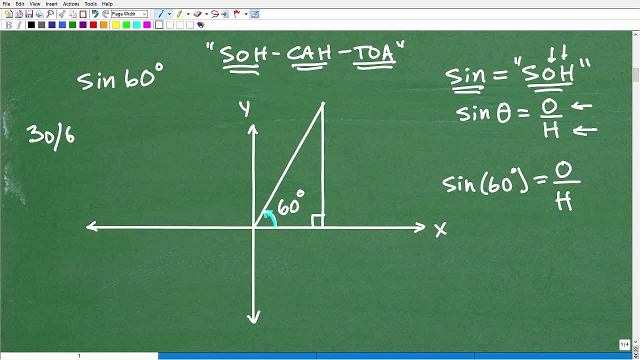 be very, very familiar with. Those are the 30,, 60,, 90 special right triangle and the 45,, 45,, of course, 90. Special right triangle. you have to know these super good. Of course, I have videos on this in. 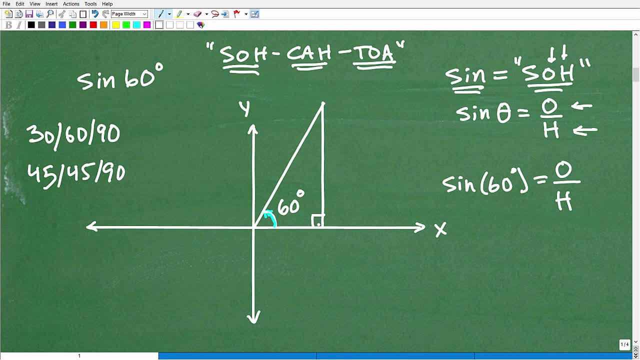 my geometry playlist as well, But in a 60,, 90, and this up here is 30 degrees right there. All right, let's put that little 30 there. You can always build a basic lengths for that any 30,, 60,, 90 right triangle. So the shortest leg of that triangle is one. 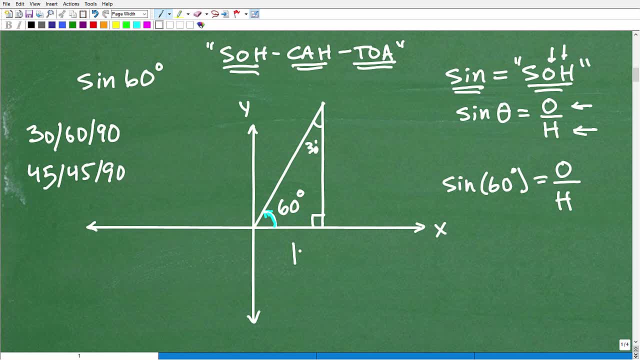 Okay, the hypotenuse is always double the shortest, So let's have this as a positive one, because we're in the first quadrant here. So if we double this side, this will be two, Okay, and the 30,, 60,, 90,. if this side, for example, 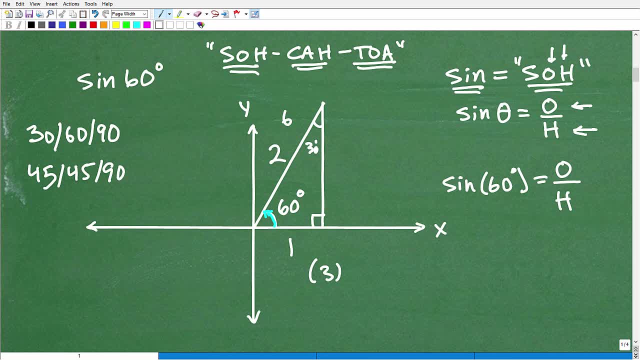 was three, then this would be six. Okay, So here I'll just do. I'll use the basic numbers here first. So this is one, two, and now this is going to be the square root of three. it's actually. 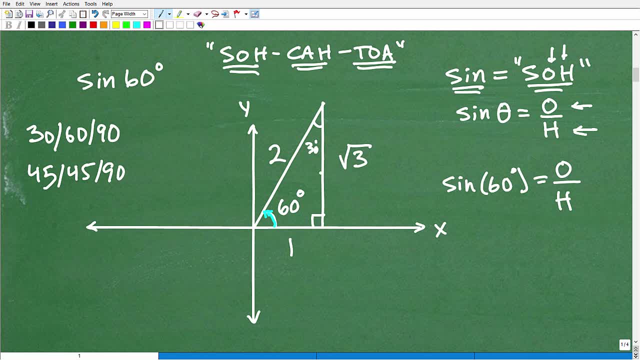 one times the square root of three of this length. Okay, let's do another. I'm going to put these, the values here, but let's just do something real quick. What if this was three? Okay, the hypotenuse would be double that, So that would be six. And then this side, this medium side of the 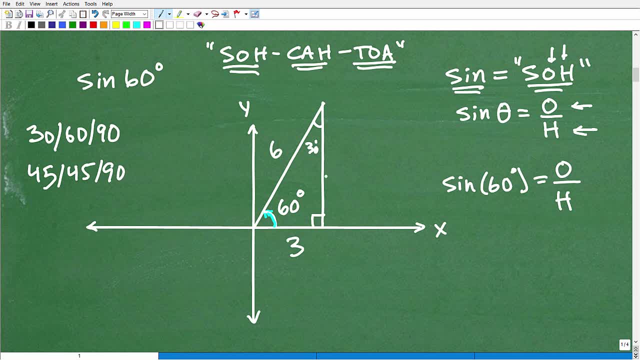 30,, 60, 90 would be this side, the shortest side times the square root of three. it's always times the square root of three And this is always the shortest side, right there? Okay, All right, so you got to understand: 30,, 60,, 90,, 45,, 45 special right triangles. that's critical to your success. 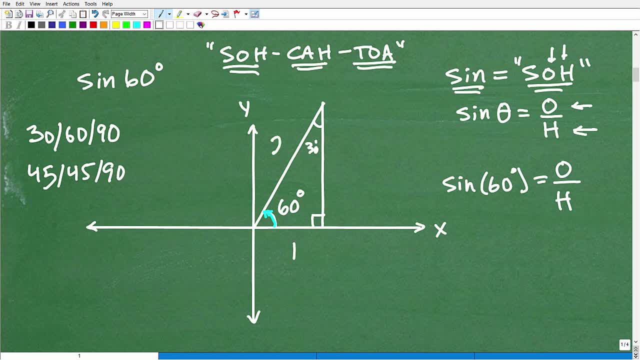 with that. But let's go ahead. Put some basic numbers in one: two square root of three. Now, when you're doing this, if these angles were in this quadrant- the second or third or fourth quadrant- you're going to be very 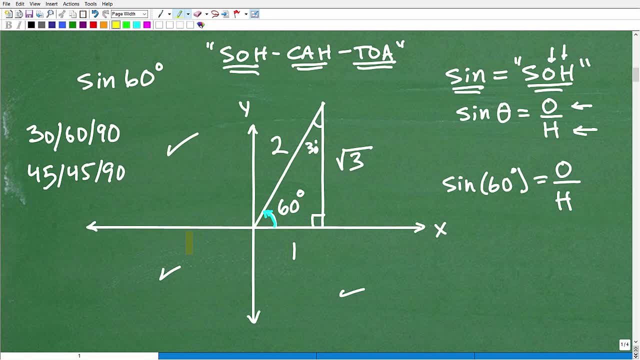 mindful that you know this. these are going to become negative. over here You got to understand the values- positive, negative values- of these legs, of these triangles Here. this is positive one on the X axis and this is positive on the Y axis. Okay, And of course, 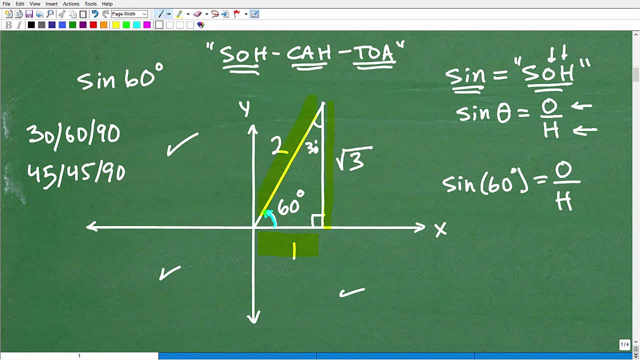 the hypotenuse will always be positive. Okay, All right. So now we got ourselves some actual measurements of this 30,, 60, 90 right triangle, So now we can actually go ahead and plug them in for the opposite over the hypotenuse. So, sine of 60 degrees, our opposite, is the square root of three. 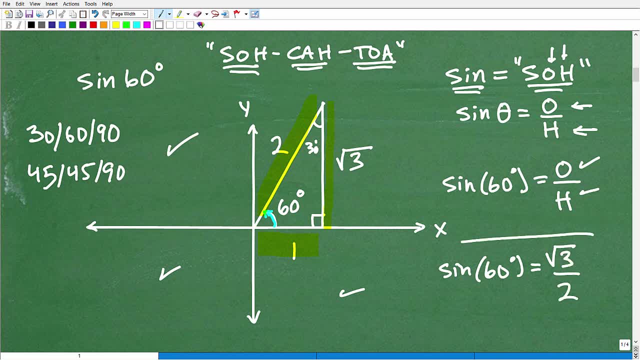 and the hypotenuse is two And you are done. That is the answer. That's the exact answer. Now, if you want to just kind of, you know- prove that to you, go ahead and take the square root of three and divide it by two. 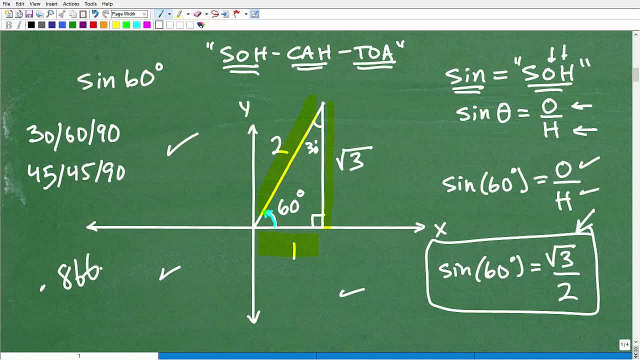 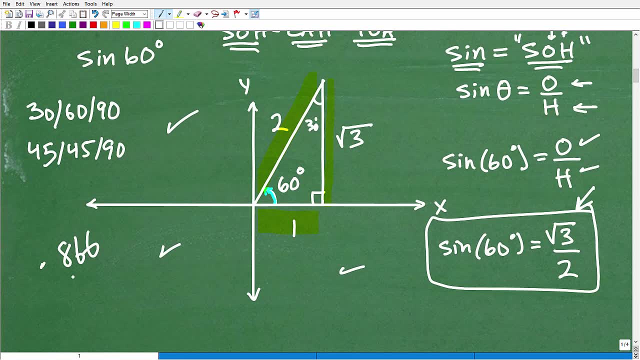 I guarantee you you're going to get that decimal 0.866 or whatever the case is here. I believe that's what it was. It has 0.866 that we kind of already, you know, had as an estimate on that. 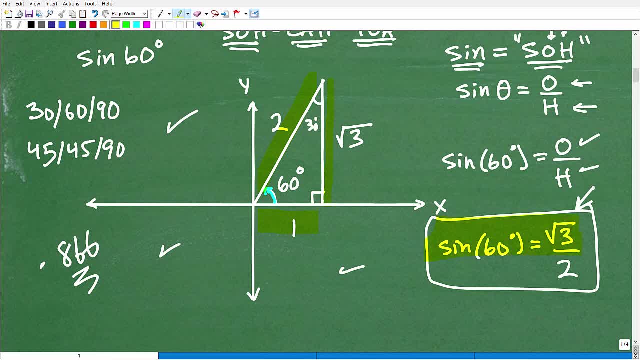 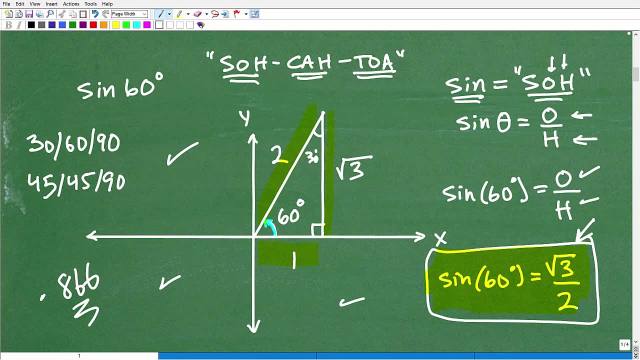 sine graph. Okay, But this is the exact answer that you want to know. So this is about, again, a pretty basic illustration of a skill that you need to have in trigonometry, which is to be able to evaluate the value of the triangle. So this is the exact answer that you want to know. So this is. 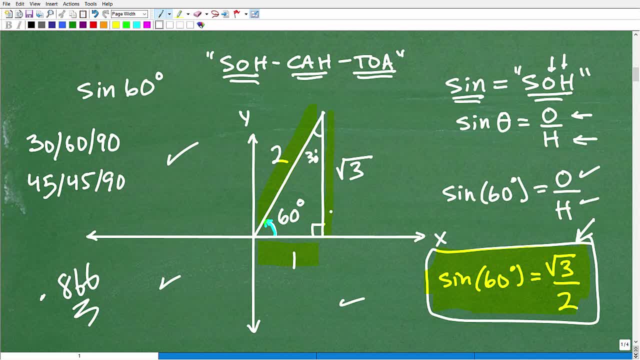 the exact answer that you want to know. So this is the exact answer that you want to know. So this is trigonometric functions for these very, very common angles. You have to know how to do this, And it gets more sophisticated when you're dealing with radians and angles in this quadrant. 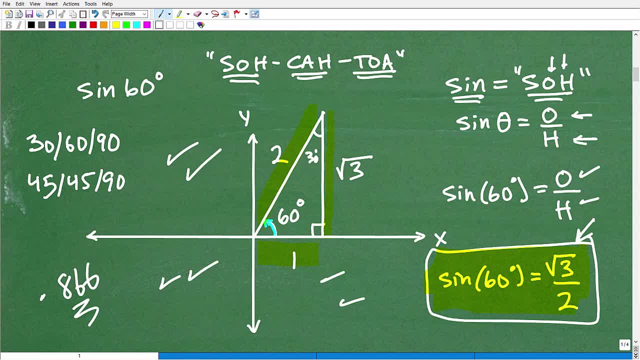 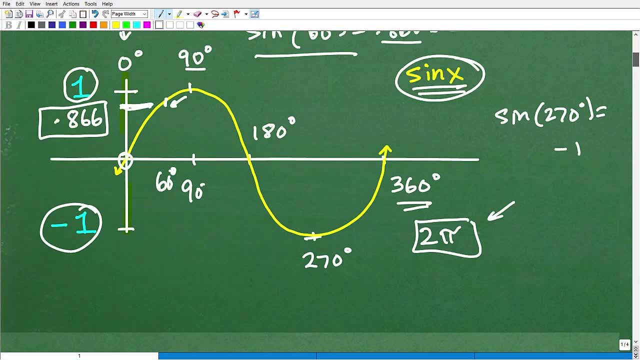 this quadrant, this quadrant. You got to get really really good at this, Okay, And hopefully now you're like: okay, I understand this. If you understand this, then you're going to be well on your way of understanding all the other problems as well. But it's always nice to tie in. 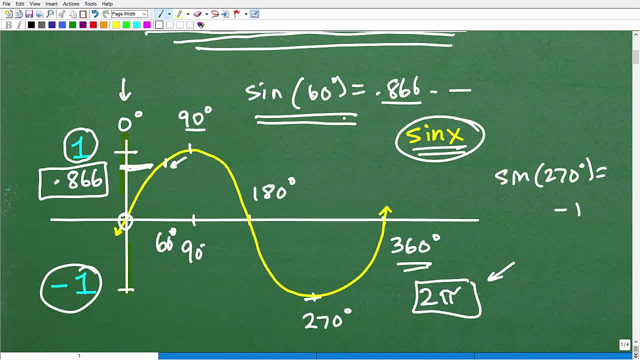 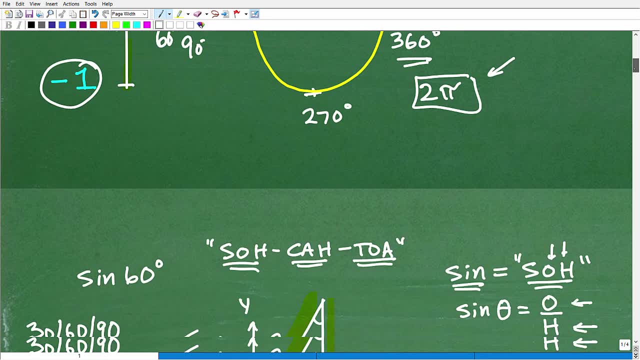 your work with these graphs, or trigonometric functions. You know, Try to make these connections the best you can. And if you think about it, you know this graph and all this information that I covered with you here today. how could you possibly, you know, do your work if you weren't? you know, taking notes. 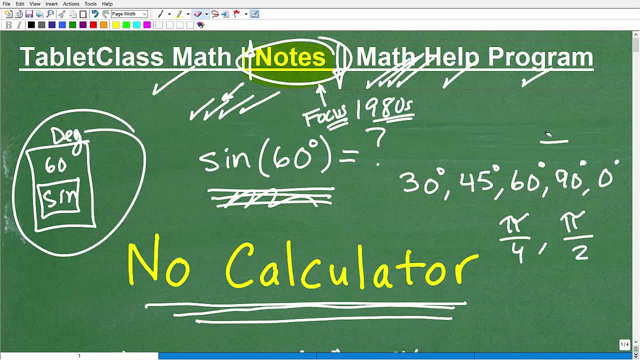 You can't be like: oh I, you know, I remember that from class. What was that again? No, you got to write. you got to write stuff down. Even though a lot of this stuff is in your textbook, you have to write it down because that's the way it's going to get to kind of soak into your brain.